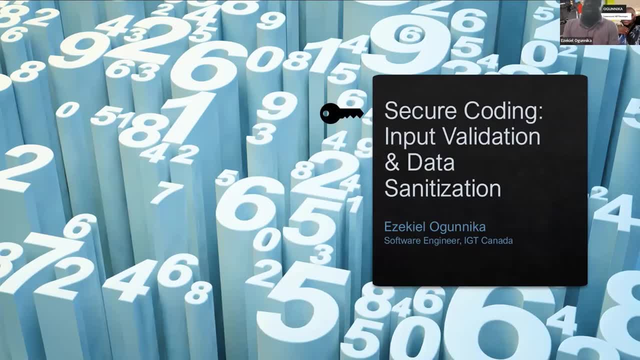 And the topic assigned to me basically is secure coding, input validation and data sanitization. So, like you all know, my name is Ezekiel Ogunnika. I'm a software engineer. Basically, I specialize in NET, So that's more of like my core strengths And I currently work. 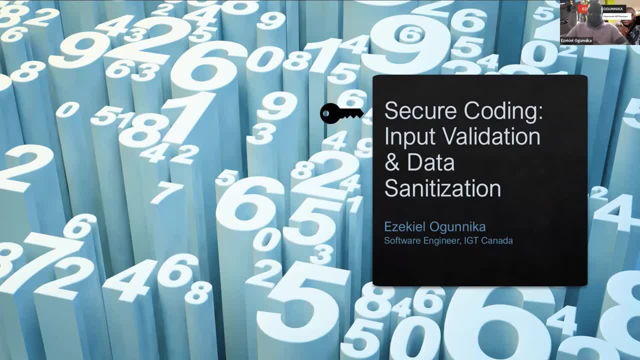 with IGT, That's International Gaming Technology. It's one of the leading gaming companies in the world And I'm in the Canada branch And that's where I work with the Lean Gaming System. So now, before I proceed, I always like to start with this very 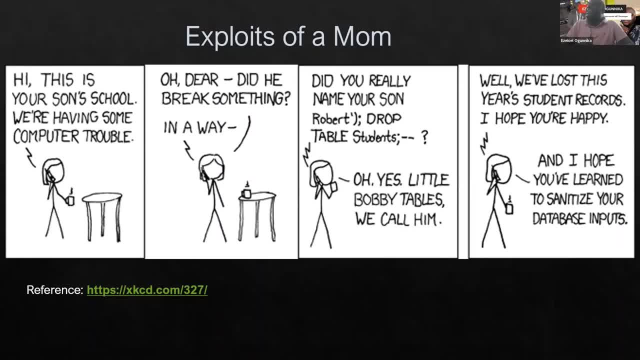 popular joke I'm sure most of us must have actually seen it. It's called Exploits of a Mom And it's a very interesting joke when security is actually validation or input validation when it comes into topic. So this is just like a. 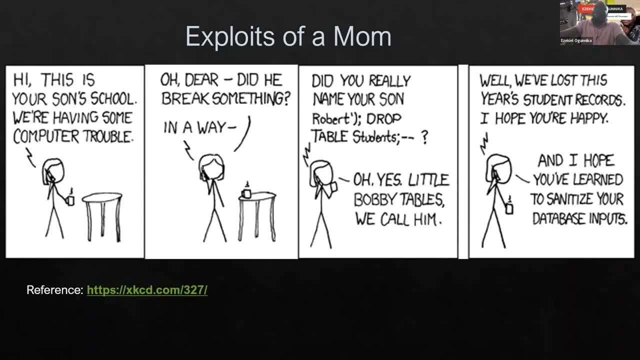 conversation between a school teacher where a call came in and this is the teacher was like: oh, this is your son's school, We're having some computer trouble. And the mom replied: oh yeah, did it break something in the way you know? And the school authority or whoever, 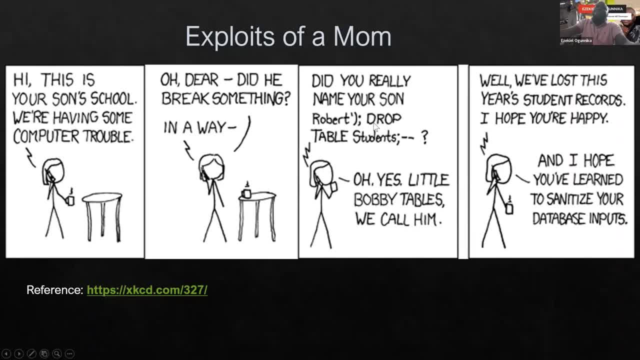 calls from the school was asking: did you really name your son, Robert or something? And the coach single quotes, brackets, semicolon, drop tables students with a comment, Oh. and the mom was like: oh yeah, this is Bobby Tables, right, We call him. Well, this admin was. 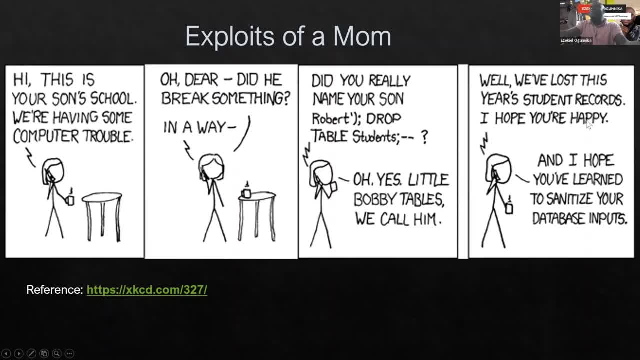 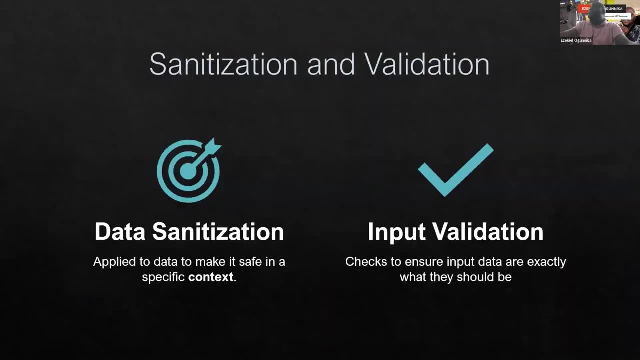 like: well, we've lost this year's students record. I hope you are happy And the mom's response was: and I hope you've learned to sanitize your database input. So basically, this actually summarizes what we'll be talking in here today: the importance of input validation. 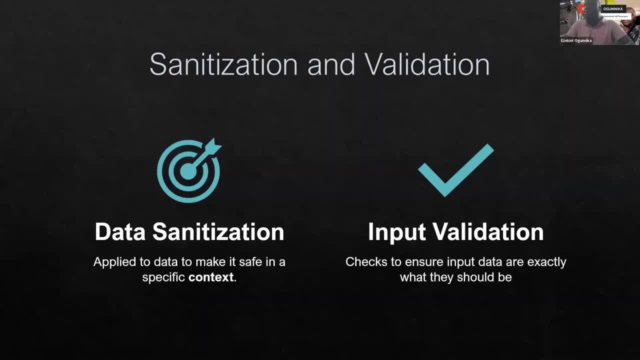 I broke it down into this: sanitization and validation itself And the two key points here. it's just a summary of what this actually entails. You know, when you think of data sanitization, the first thing that comes to mind is: this is applied to how you make a data save in a specific context. 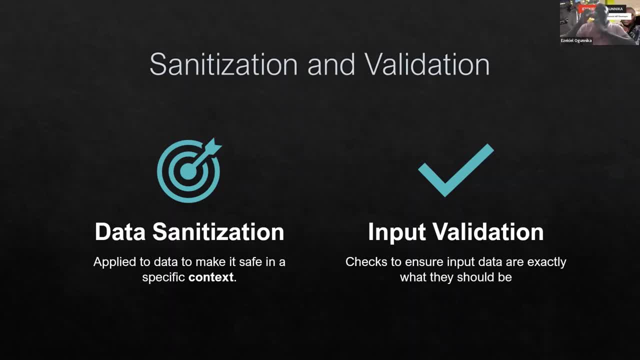 And the key word to this is actually context- Whereas input validation on its own side is actually checked to ensure that input data are exactly what they should be. You understand, they are exactly what they should be. So, in a more sense, what this actually means is that validation itself is concerned with making sure your data is actually valid. 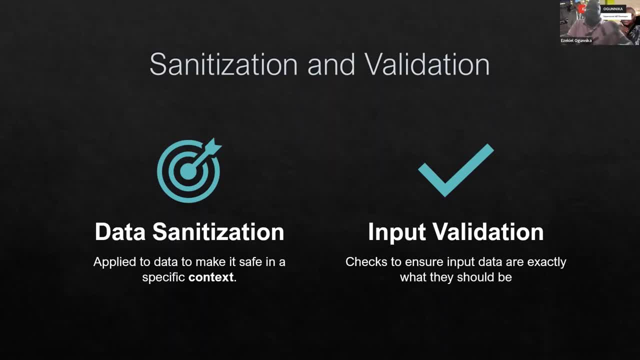 And data sanitation itself is about making it safe, Why some of the validation might be useful in making sure data is safe right In general, it is not sufficient. So even when data is valid, it might still be unsafe in certain contexts as well, too. 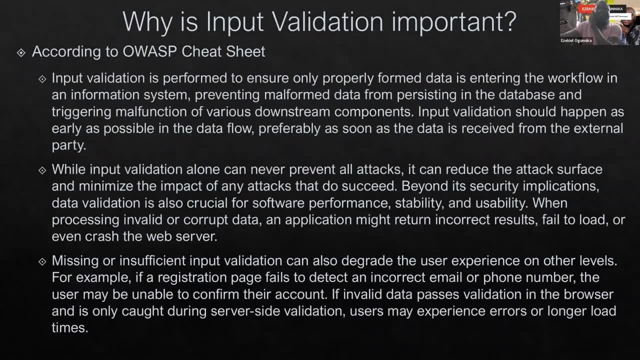 And this takes me up to the next slide itself- And mostly everything you need to know about validation is actually well-detailed in the whole app's cheat sheet, And I think I wouldn't have been able to pull this off without making reference to the whole app's cheat sheet in this regard. 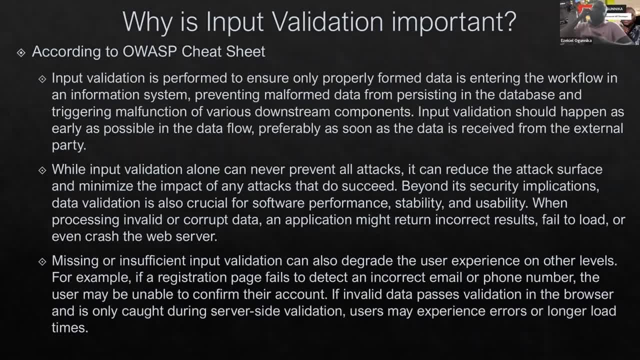 So why is input validation itself, Why is it very important? right, And it says according to the whole app's cheat sheet, input validation is performed to ensure only properly formed data. It's entering the workflow right And entering the workflow in an information security, preventing malformed data from persisting in the database and triggering malfunctions of various downstream components. 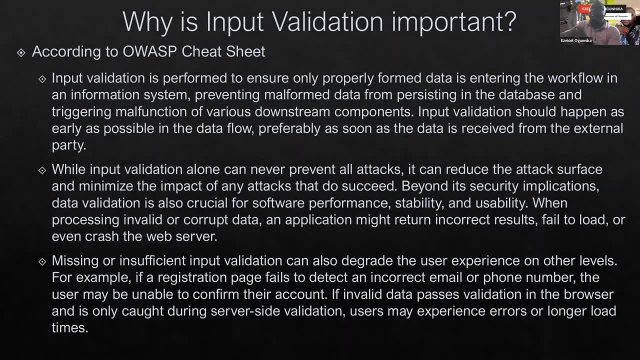 Input validation should happen as early as possible in the data flow, preferably as soon as the data is received from the external party. And I think this is where it's very, very key for us as developers, right? Because when you think of security, the very first point you take. 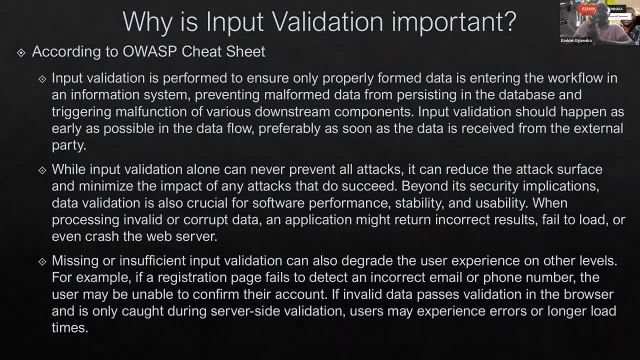 What you think of is, before you start talking about infrastructure, network, networking, security, you first start to look at the application itself. So the very first part of any solution out there or any system out there itself starts from the developer itself. And I think this is a lead tool we can contribute, because in your sense we are not security experts somehow, but we still also try to be experts, adding that to our role in what we do. right, 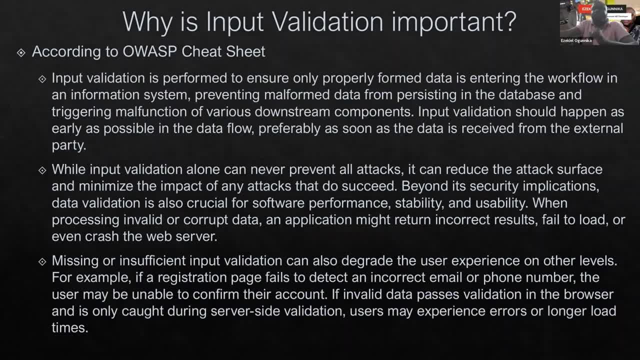 So why is it important? Why is it important? Why is it important? But the high-level validation alone also- This is also a point that is very important to note as well too- that can never prevent all attacks. It can reduce the attack surface and minimize the impact of any attack that do succeed. 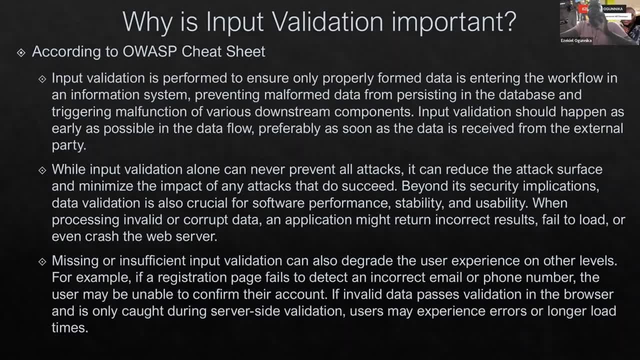 Beyond this security implications, data validation is also crucial for software performance, stability and usability. When processing invalid or corrupt data, an application, by returning correct results, fails to load or even crash the web server. missing or insufficient info validation can also degrade the user experience on another level. 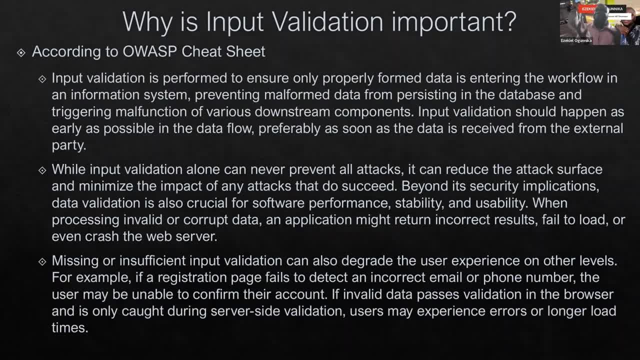 and i also try to put this also for me from i as a developer. most times i try to put myself as a user: and what do i expect? what do i really want? so and i- this is a typical example- right, if your registration page, for example, fails to detect an incorrect email or maybe a phone number and the 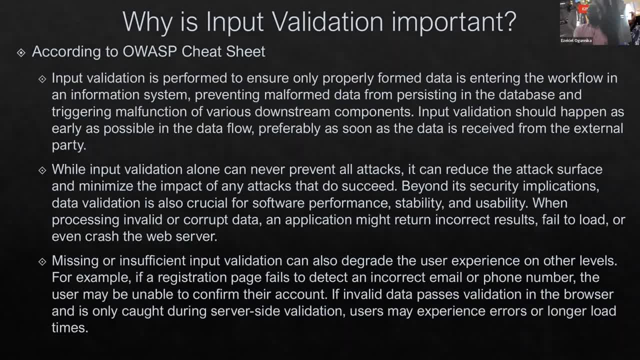 user was unable to also confirm the account. so what's the purpose of me coming up to your site? i want to sign up, i want to enjoy the services i put in my email, but because in the process i- i there was a little typo, maybe it's space at the back that wasn't trimmed and i have it stored as. 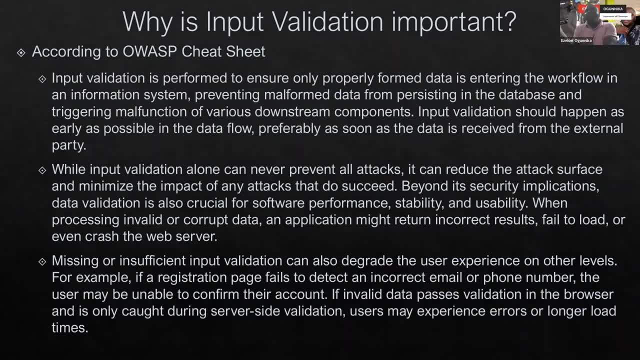 it's supposed to be. and each time i keep putting my email the system keeps telling me maybe one part of the system itself keep validating it with a trim um text and the other keeps validating it on trim text itself. you know it brings about a very horrible. 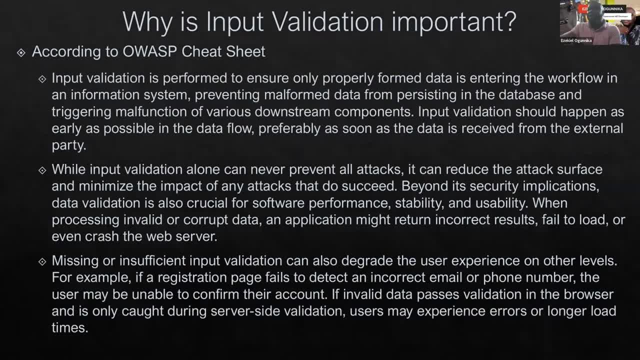 experience itself. uh, from a, from a, uh, a user's perspective as well, too, and that is why any system or application that works with input data needs to ensure that what it is valid. this applies equally to information provided directly by the user and to data received from other system. um. 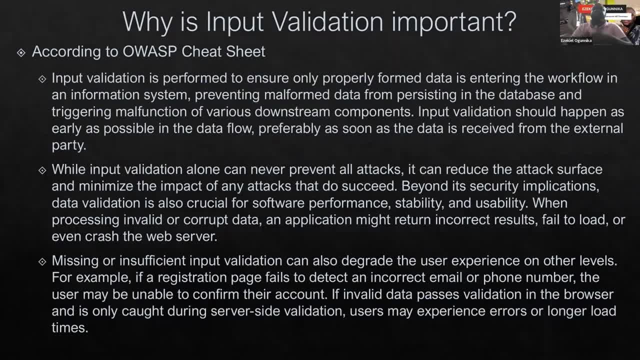 so now in web application, basically right, input validation is typically understand as checking the values of web form. uh, web form input fields, right. this initial client-side validation is performed directly in the browser in most times web. you know where you do your web validation, uh, but you also need to check what is being submitted at the end of it all. um, sorry, oh that. 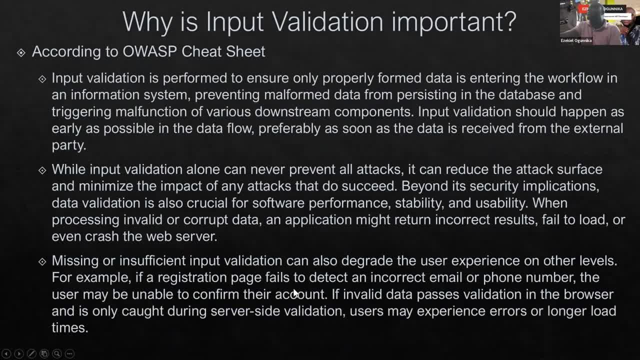 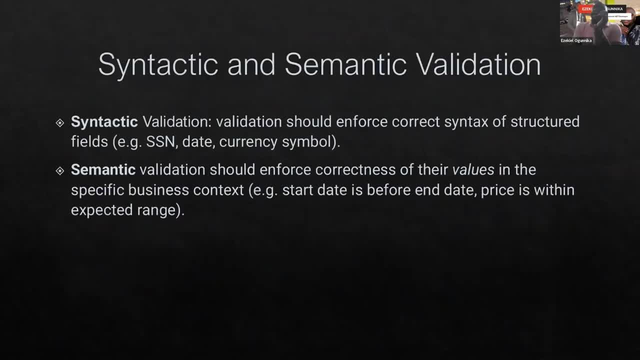 was not what i wanted to do, okay, uh, yeah, so going back to the next slide now, uh, what's happening? okay, yeah, there are basically two types of, um, improved validation. this also is available on the on the whole website as well, too. that can be done on any uh application itself. uh, the first of 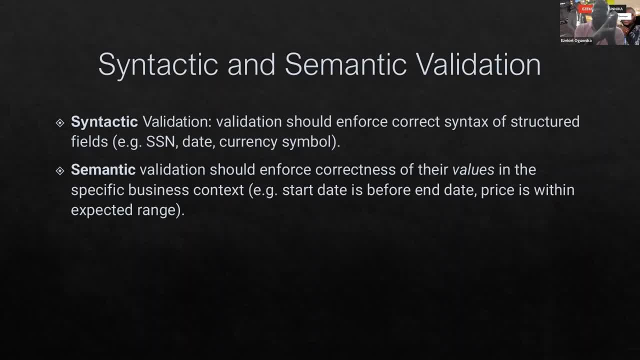 it all being a syntactic validation and the other being a semantic validation itself. so when you talk about syntactic validation, uh, validation should also ensure correct syntax of structured field, your serial social insurance number, the date currency symbol where you are expecting the currency symbol, it should always be a currency symbol, right. and when you think of semantic, 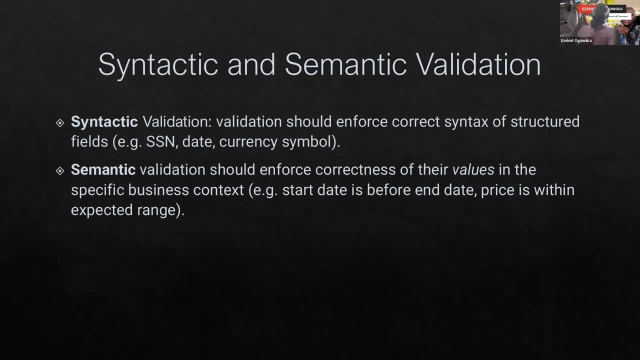 validation this time around. this should also enforce correctness of their values in the specific business context. so let's say, for example, if you have a business where you are expecting a price, for example, you're looking at setting up a, a field where a user has to put in a start date. 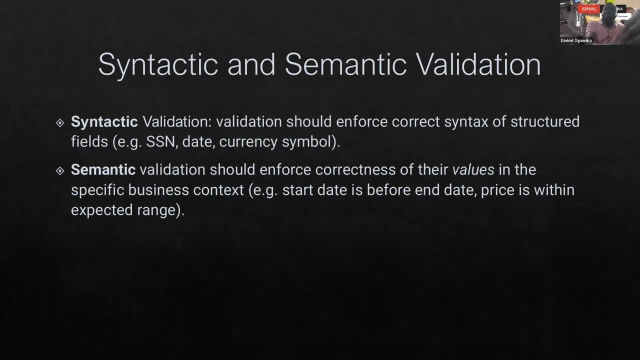 and an end date right, and a user is trying to put in a an end date as a start and putting the start date, uh, as the end date itself. of course, when you're comparing the data via range, having it flipped surely will give an unexpected result, and also in the place where 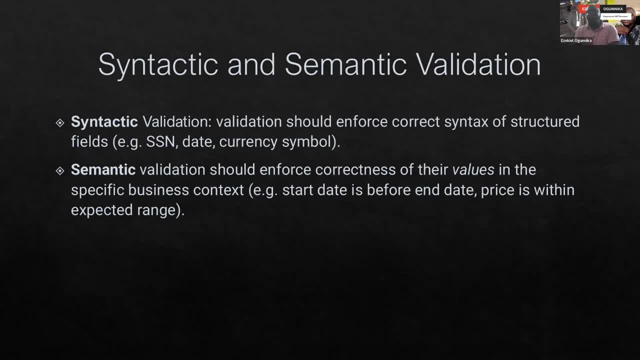 you're expecting the price a user is putting in the name of the product. you know this actually brings a lot of inconsistency right with um within a system. so an application to check that data is both syntactically correct and semantically valid as well in that particular order you check if i'm 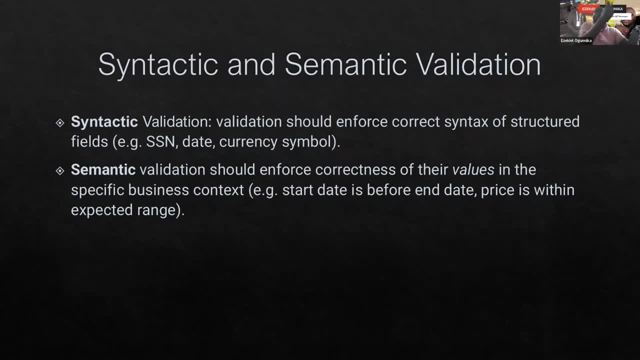 supposed to put in a bank verification number, for example in nigeria, or a noban number, which you all know is just maybe 10 characters, and the like. we should ensure that this is syntactically correct and semantically in the sense that am i putting a bvn number in the place i'm supposed to put in an? 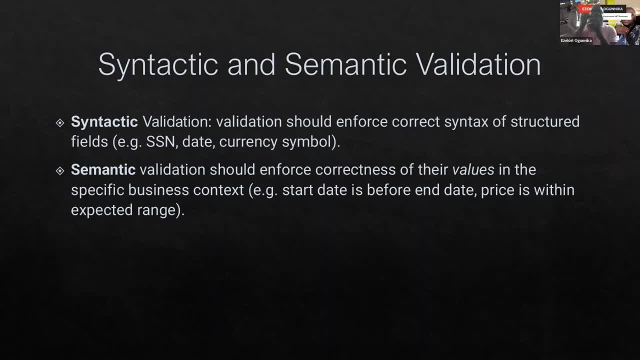 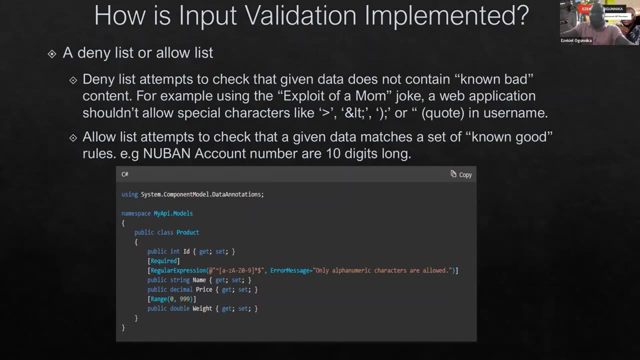 account number. do i really need to have numbers? you know, that is also another aspect we also need to look at before using it in anywhere within the system itself. um, moving on, so now we uh, according to oabs as well. like i said, this is not going to be done in isolation from the standard defined. 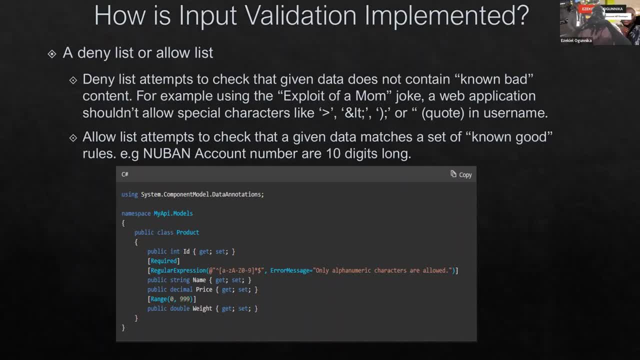 on the oab's uh page. um, so how exactly do we do input validation itself? how exactly is input validation performed from the uh developer's angle? uh, one of the approach that was stated? uh, in you have in a deny list or an allow list? um, and what this actually means basically is: 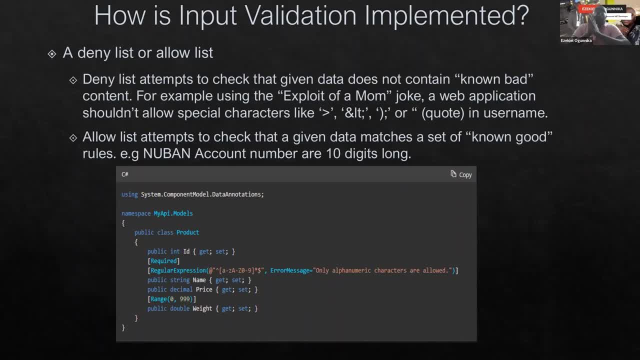 denying leaves attempts to check that given data does not contain known bad content. you understand, looking from the example of the exploit of a mom joke that was shared at the beginning of the page right. a web application should allow special- shouldn't allow special- characters like uh that. 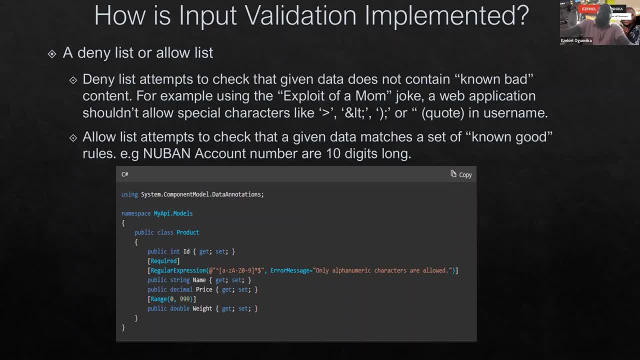 are known to basically for injections and cross um um side scripting. you know, should actually try to not allow any of these in the username. because you're asking for a username, why should i have these in my username? ideally should be pure plain text and also the other uh aspect of it is also 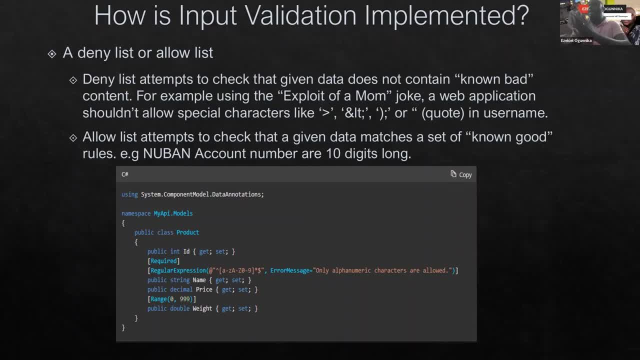 like an allow list itself, and this stems from you allowing to check that the given data matches a set of known good rules. and that goes back to the example i created when i was talking about a new account account number. we all know that nuban- uh sorry, it's peculiar to nigeria, right? it's like um. 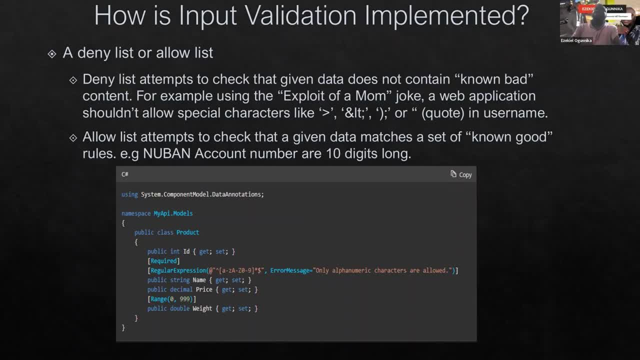 uh, it's a nomenclature agreed by the bank to say all banking account numbers are supposed to have a certain digit, and we all know that banking numbers shouldn't be 10 digits. why should an application give room for you putting in 11 digits, 8 digits, you know, or even more than what is? 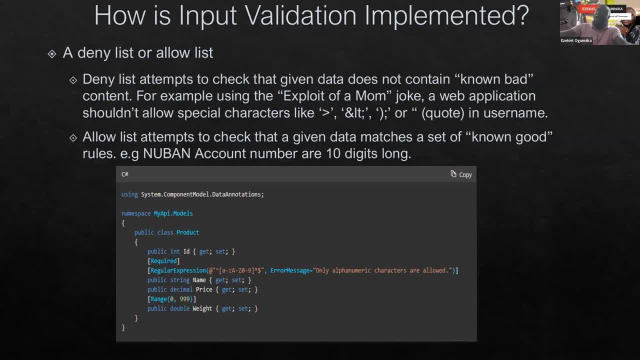 expected in that particular regard- and this is a screenshot of how some of this could actually be done, you know, uh, or prevented, using a typical model validation from microsoft, which uses an average expression and also selecting the range, you know, uh, in terms of when, when the model itself is being presented. 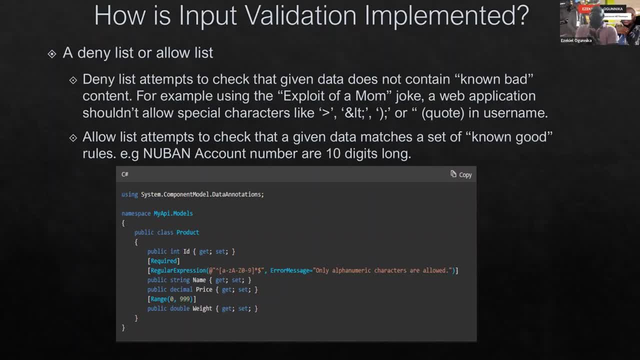 out. so when you're talking about a name, you should know names are supposed to be, only alphanumeric characters are allowed, and we're talking about weights, which should always be numbers alone, and this is one aspect of this. uh, but with this model we are trying to show uh. 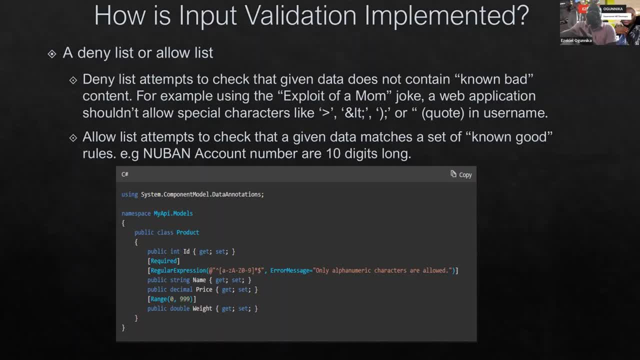 With that being said, also, regular expression on its own has some of its own exploits as well, which I think has been proven also in the past, where denial of services could also occur. you know, when you have a regular expression that is not well formed, that could actually expose your application to denial of service. 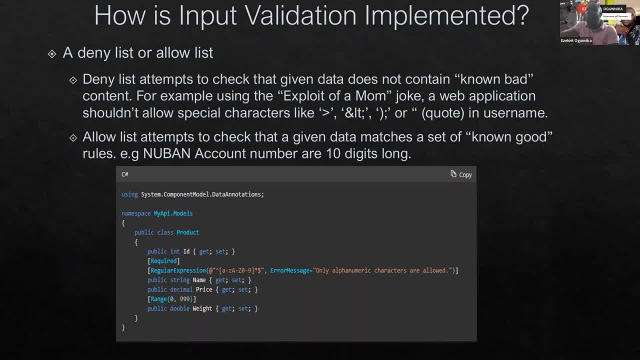 And I think one of the things Microsoft also did in particular was you having like a timeout, setting a timeout for your regular expression itself. So if I'm running a check against a regular expression, I could set a timeout global-wise within the application itself, to say: 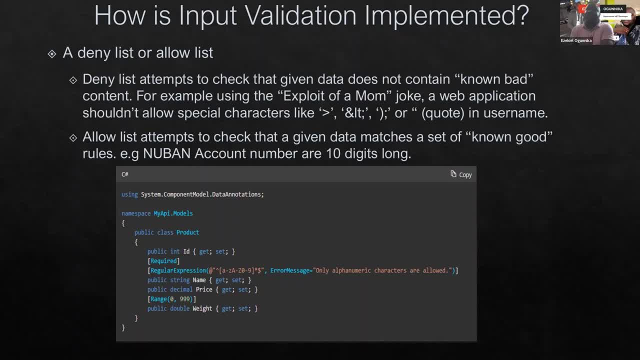 any regular expression checks I'm doing shouldn't take more than five minutes. With that you know, you're 100% sure. if there's a regular expression check for a malformed regular expression, your service is actually not going to be denied. You can't have an attacker trying to deny, do a service denial by putting in a test against your validation. basically, 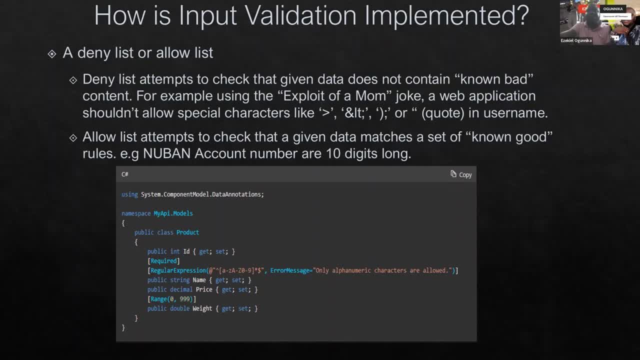 So what Microsoft did in that regard is: you have like an attribute that you could set a timeout limit within your app config or within your web config, And for those into cloud these days as well, too. on Azure, you can also get this done as well by having a configuration value. 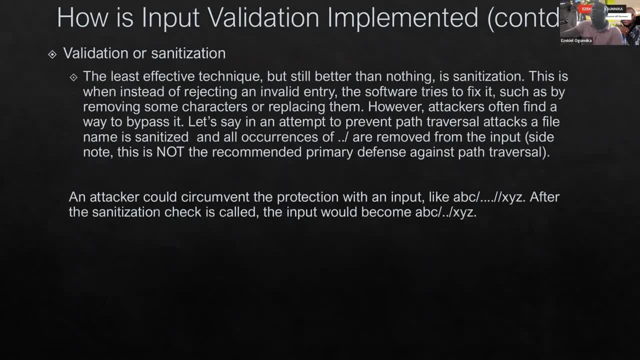 for regular expressions. that's not going to be beyond that. So now also, the second way of also getting this done is by validation or sanitization right. So this is also been proven to be like. this is similar to what Glenn showed in terms of when he was talking about document traversal. 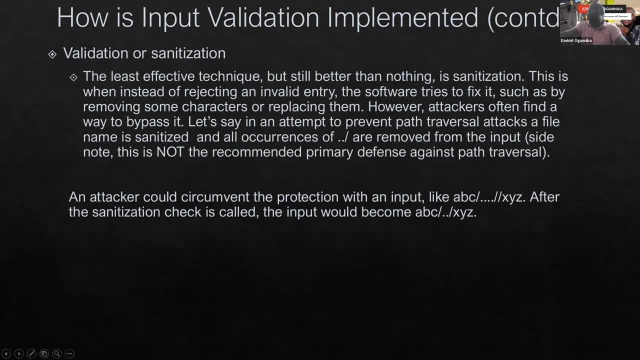 or file traversal, basically like ESD, in which he did justice to me in that regard. right, So sometimes we are developers, we try to fix things right. You know, we try to like okay, instead of rejecting an invalid entry, let's try to make it work. 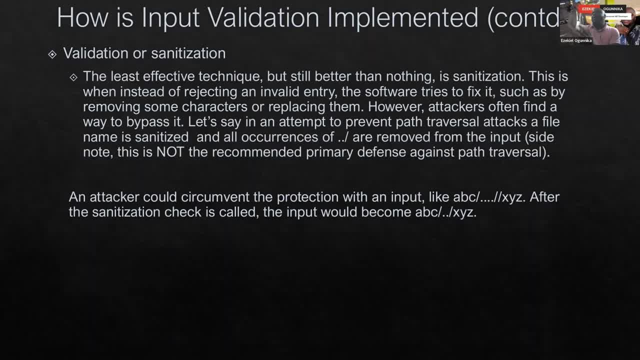 Let's try to fix it, Like the example he showed, where we in file traversal, where you're trying to replace every dot with a forward slash from every file name that has been passed, You know. he showed us also a very typical example- what I also have listed here- how this can also be circumvented, right. 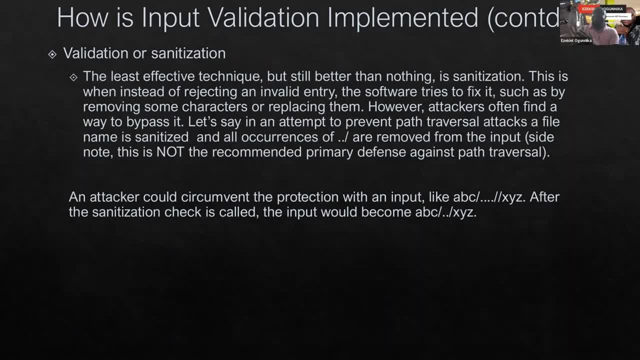 So, in the real sense itself, you, if you're looking at maybe after validation and sanitizing to an extent you probably have to, don't really take it too personal when it comes to as a developer. you know you want to be sure your application does everything you've done, but like the typical example you showed. 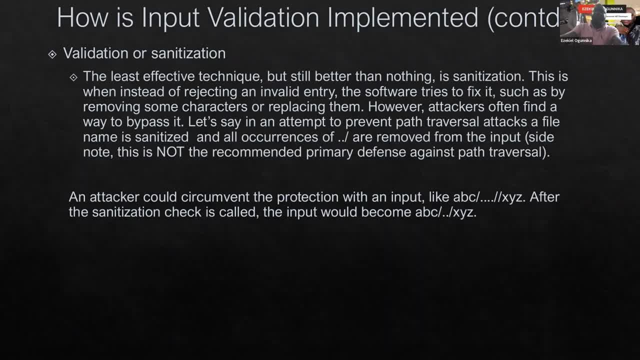 since we know that this can actually be done at very points during your validation and sanitization, you can decide that it's okay. yeah, I know I've replaced this. I'm having the local variable itself showing the right part that I want it to be. 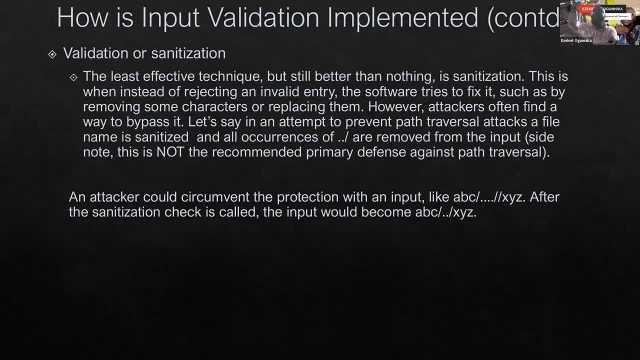 If it's going to be in a text folder, ensure it's actually pointing to a text folder And with that aspect, right. if any other thing doesn't fit into what you have in your code, which sometimes people might say, oh yeah, but like why not just try to fix it? you know, get it done. 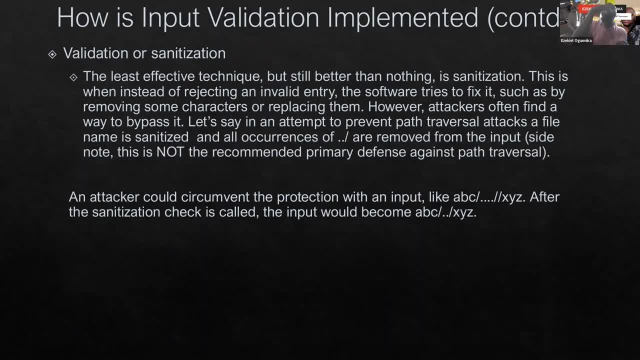 Let's see how many times you can loop over the after searching for a double backslash, search for a double forward slash. you know, sometimes it becomes an overkill in the real sense in that regards. So another thing also that I want us to know here is we shouldn't confuse this validation right. 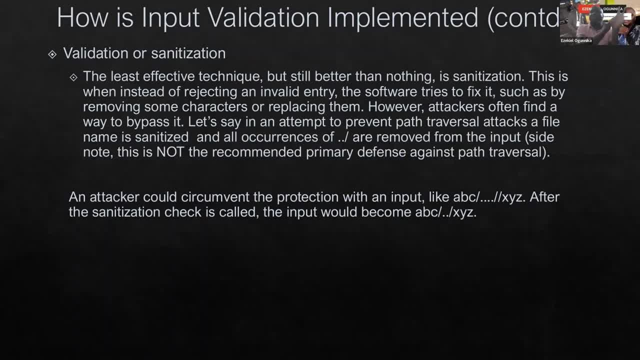 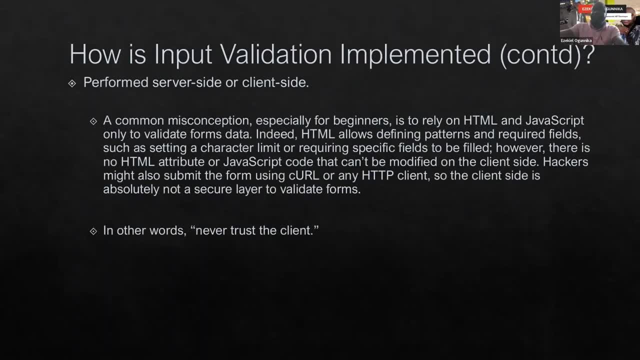 to data sanitization, So that we talk- which, like I said, it's a context- we'll surely get into that in the subsequent slide as well too- And one other way also of doing input validation. basically, is you doing a server-side or deciding between a server-side or a client-side validation? 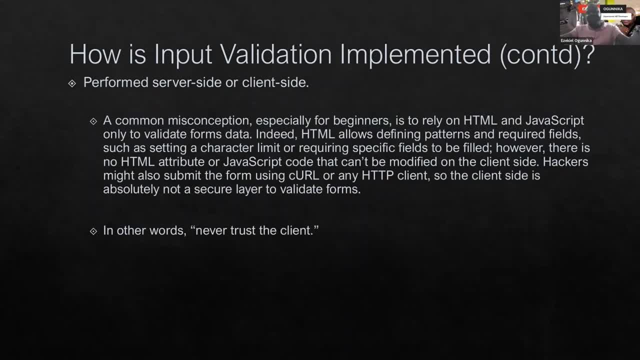 You know, these days now we have lots of client-side development frameworks out there. you know we try our best also in bringing user experience to the right way, that we think of, you know, giving you the right dialogue, but most times right. 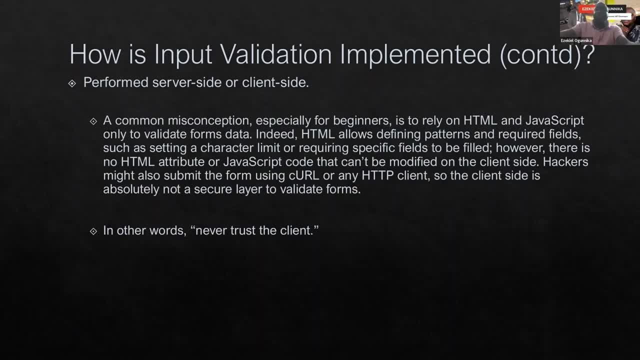 the bottom line is you should never, always, trust your clients, no matter how robust they are. Don't trust your clients. Anything could have happened and you don't really have the control over right. Always ensure you do a server-side validation. 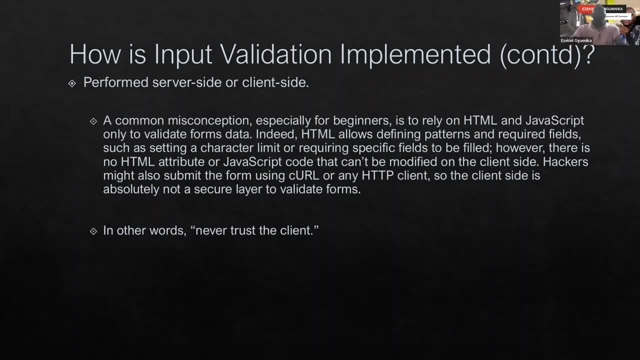 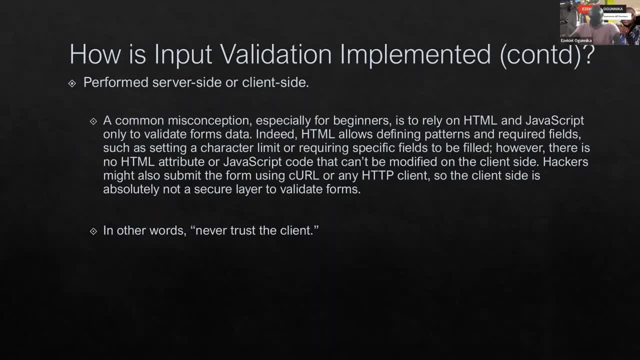 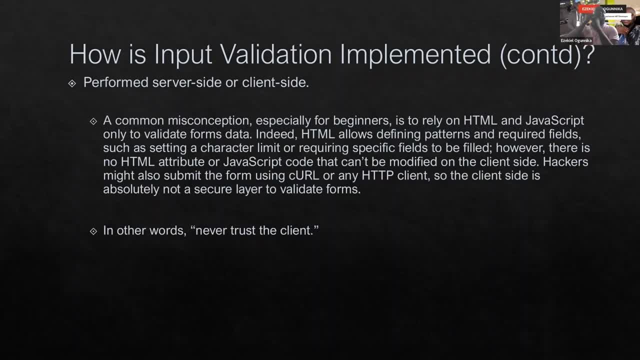 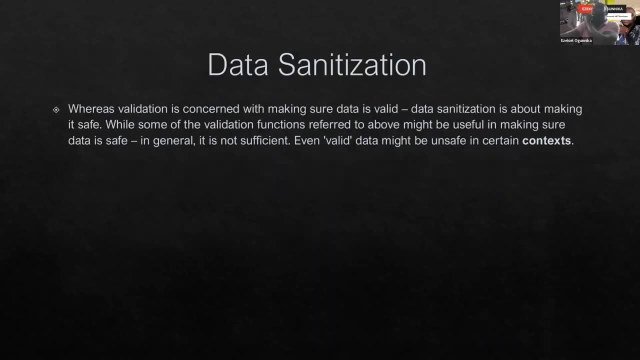 The client side is actually not a secure layer to validate. So, like I said, the bottom line is: don't always rely on the clients. By the time you get to the server end itself, ensure validation is also done at the server side of your scripting as well. 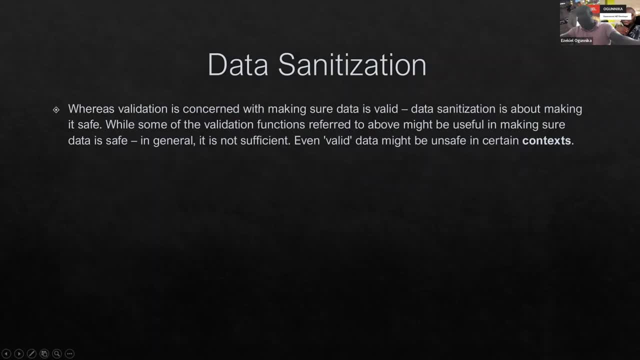 And that takes me back to- and I will give you some more details on that- to the sanitization aspects of this, of this topic itself. um, and what basically happens here is um. whereas validation is concerned with making sure data is valid, right data translation is about. 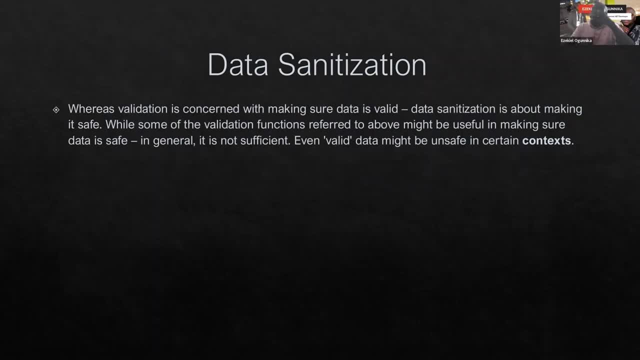 making it safe and i i think i i gave an uh, a context to this earlier right and one of the, the prone, or more of the common um uh, danger of, you know, sanitizing data. basically like uh, because you feel you've done an input validation right, your input is valid. 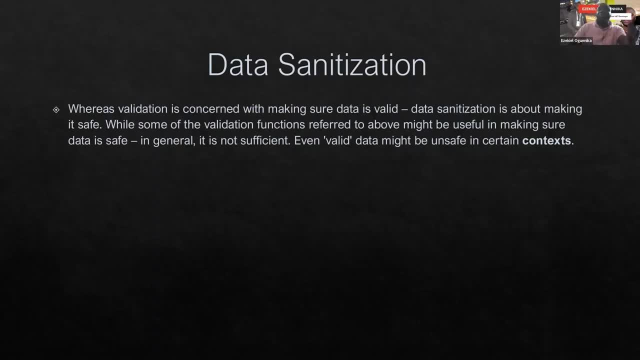 but the whole concept is, what you see is actually not what you get. when it comes to data sanitization itself, you can. you're looking at the text. it looks: oh yeah, it's valid, it has the right store, it has the right details itself. but does it really mean that the fact that it's 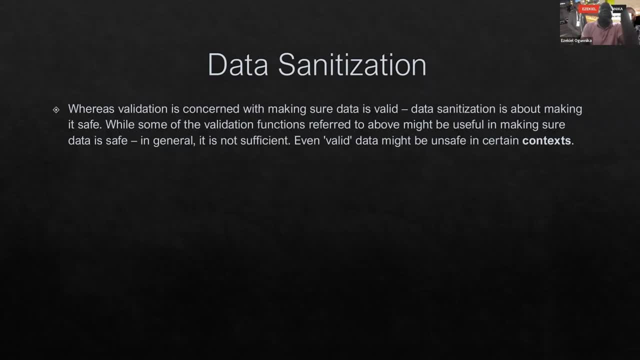 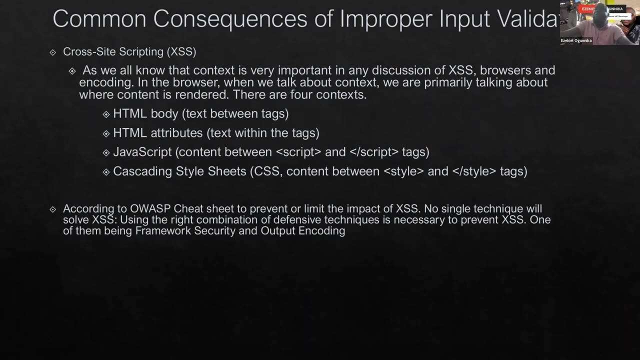 valid where it's supposed to be? uh, when the information has been done, does it really mean it is saved in a different context itself, and that's why we have to go back to come on, we have to go back to the first part of this talk about: um. you know the consequences of uh. 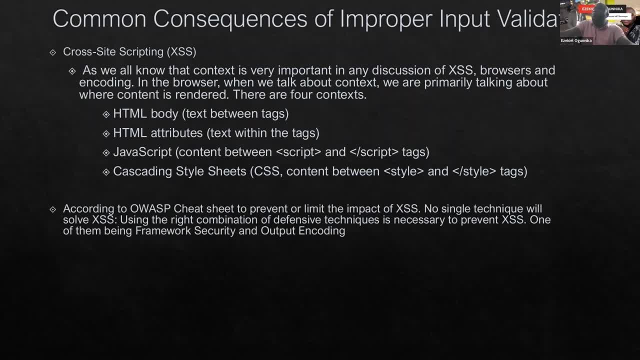 improper input validation. like we all know, um cross-site scripting, um, it's one of the um uh common uh attacks that are actually out there. you know, i just created value which enables an attacker to play some client-side scripting, usually javascript, right into web pages and when. 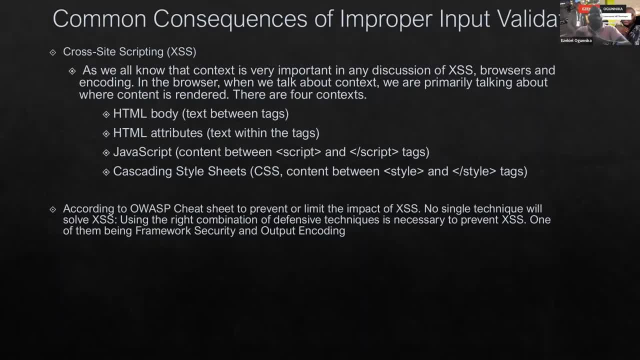 other users load these pages right. the attackers can run their screen, do whatever it is still. cookies change the content of your web page. you understand true dumb manipulations or redirecting the browser to another page. several xss vulnerabilities generally occur when this application takes user input or output into a page without validating or basically without doing. 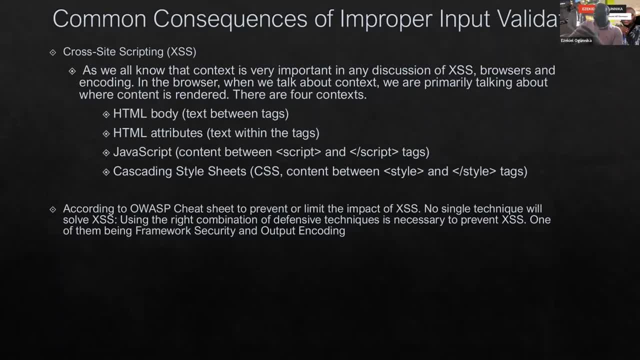 encoding, which we're going to get into also in details. so like, as we all know that context is very important in any discussion of cross-site scripting browsers and encoding in the browser, when we talk about context, we're probably talking about where context is being registered, rendered. 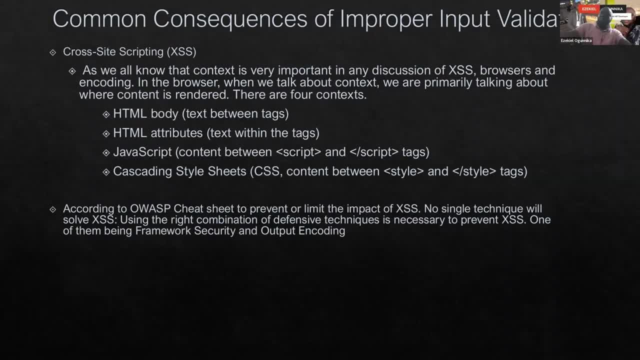 rather, there are four contexts in a typical web application. you have your html, body, html attributes, javascript and, of course, your css as well too, and according to oapps chitchat to prevent or limit the impact of xss, it has been proven that there is actually no single technique to solve cross-site. 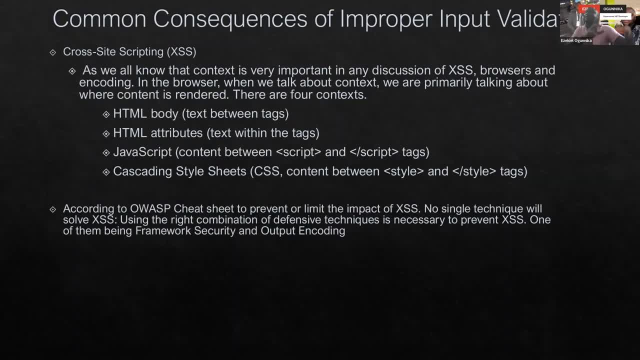 scripting. so, with the right combination of both, defensive technique, right to prevent the xls, one of them, actually one of the recommendations also is to use, depending on the framework, security itself and, like i said for me, from the dot net side of it, right, microsoft did a very good job. 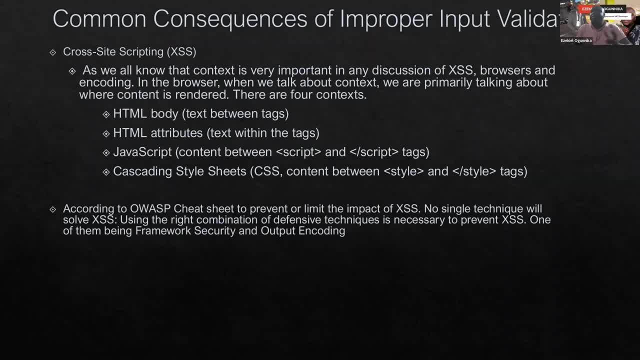 when it comes to how best you can prevent cross-site reference scripting, rather in your application, and the framework does a good job, job to that which by technically means that you can prevent cross-site scripting rather in your application. i can see that it's limited, so we will see how we can prevent cross-site reference scripts. 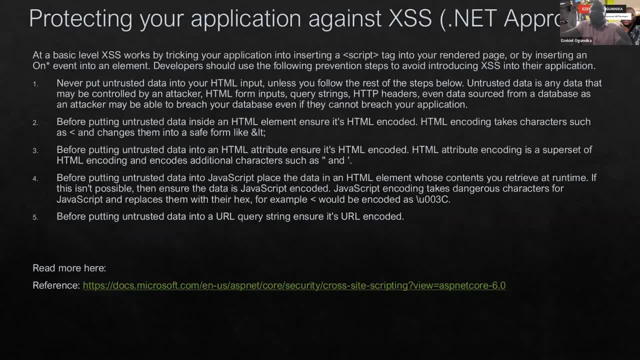 we'll get to the next slide, we'll surely see how we can have these prevented, okay, yeah, so let me go to some looking at how we can do protection, protecting your application against xss, xss, rather from the dot net approach itself. and this is actually like an excerpt from: 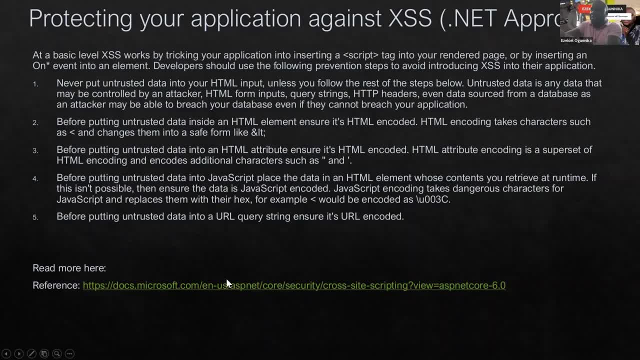 a proper documentation from microsoft and there's a reference there which i can share also. later on, instead of the basic level process, i'm going to show you how to do that. so first of all i'm going- scripting works can be tricky by your application- into inserting a script tag into your rendered p. 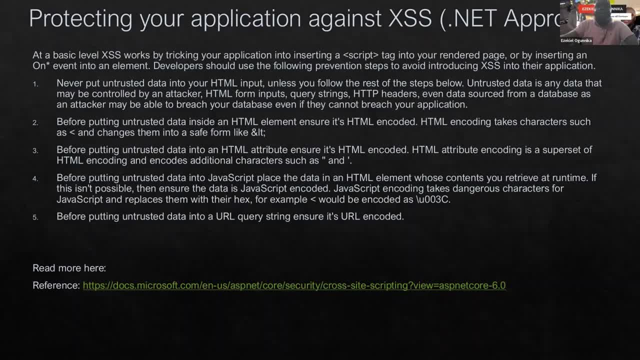 or by inserting an uh event into elements right. developers should use the following professional steps to avoid sss into the application. number one: never put untrusted data in your html input unless you follow the rest of the steps above, like before you even bring that um html values right. you first thing first is: untrusted data is in any data that may. 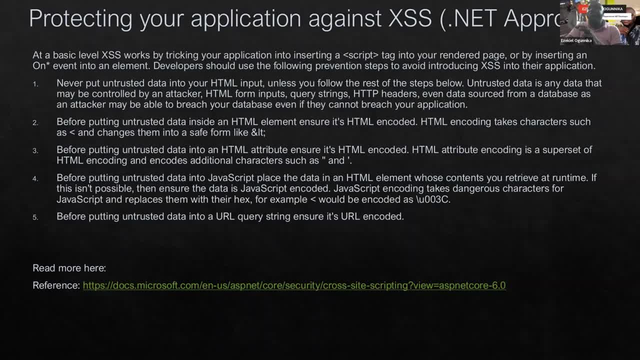 be controlled by an attacker. html form: input your query string, your html headers, the data source from the database, and i can also be able to breach your data also, like if there's a database breach and you're ready to solve, an attacker might have breached your database as well, and by 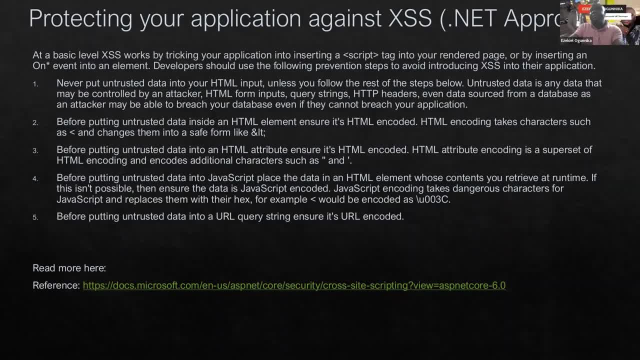 time you're running some of these onto your application, whatever it is the intention of the attack is can also be executed, and the step says that, before putting untrusted data inside an html element, ensure it's html encoded. html encoded including text characters such as a scripting tag, and changes them into a save form like this: uh, can. 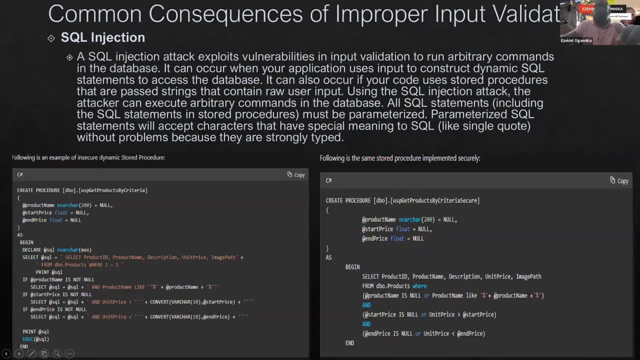 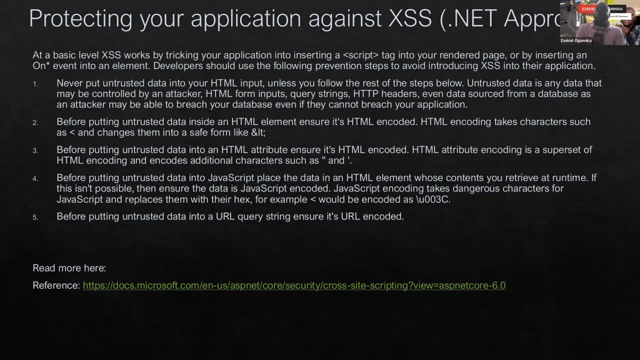 you see what i have a light idea, like the odds- oh, sorry about that, i'm not clicking- takes me to the next page. and also, before putting on trusted data into an HTML attribute, ensure it is is also encoded html attributes. encoding is a superset of html encoding and includes additional. 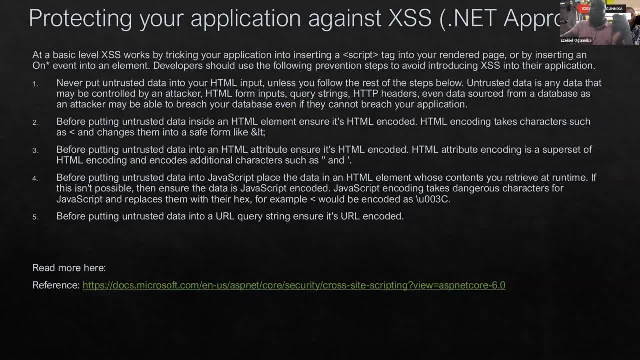 characters such as: and you know. and also before putting untrusted data into javascript: uh, javascript places data in an html element whose content you retrieve at runtime. if this is impossible, then ensure that data is javascript encoded. javascript encoded takes dangerous characters for javascript and replace them with their x and xml version, for example, a greater. 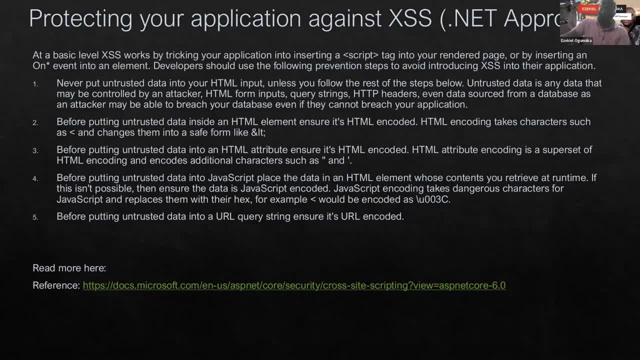 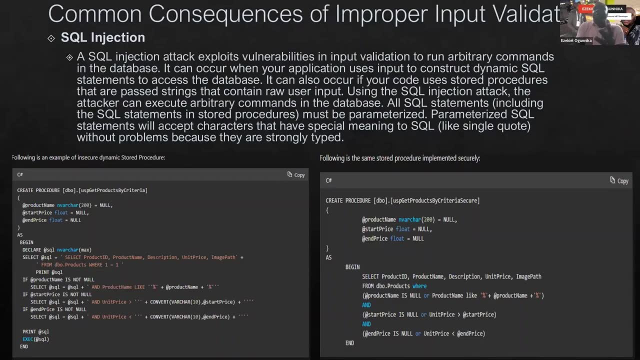 than will also be encoded using this as well. then, before putting untrusted data into your url query string, ensure it is url encoded. for more information on that. you can actually get that using this link, which i can share when inside the slide itself is being shared, and also another. 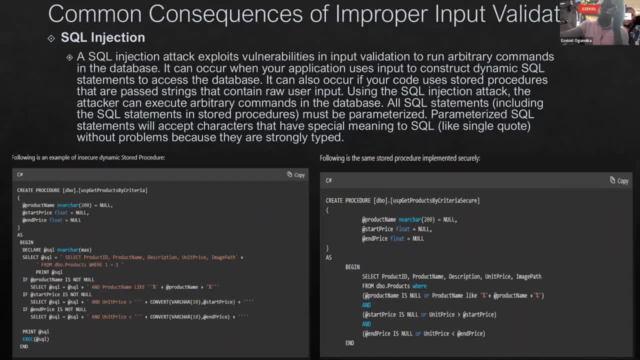 consequences of you not having the proper input. validation is one like which has been over emphasized as well, too is sql injection. you are prone to having an xml injection attack. even proper validation is not being done as well, too right, and what exactly is sql injection? it's just an attack. 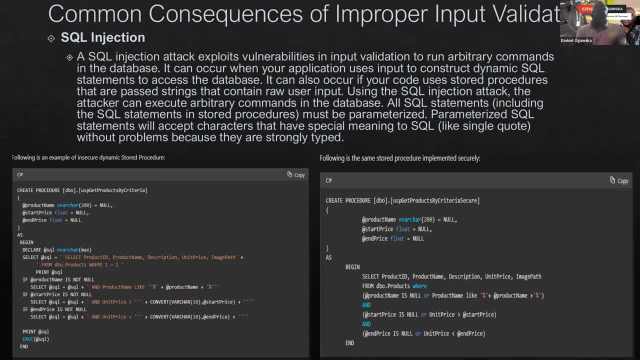 that explores variability in your input validation to run arbitrary commands in the database. it can occur when your application uses input to construct dynamic sql statements to access database. it can also occur if your code uses stop procedures. now you know, there's always this concept. oh yeah, by you going the route of stop procedures, you are, you're, you're saved. 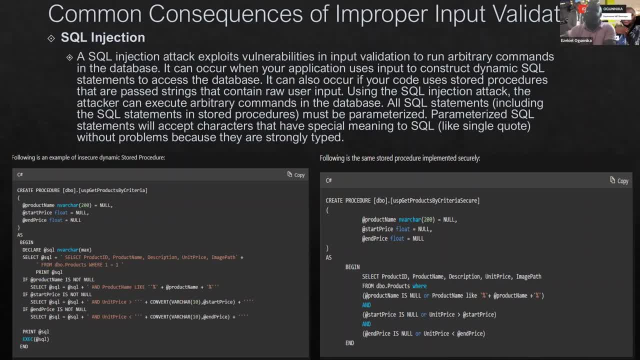 right, but what exactly do you do in your procedure? also, the fact that you're using a stop procedure to access your to do your db queries, your, your code operations in your db as well, too, does that still mean what you're practicing in your stop procedure itself? does that still make it save as well for the data that you're? 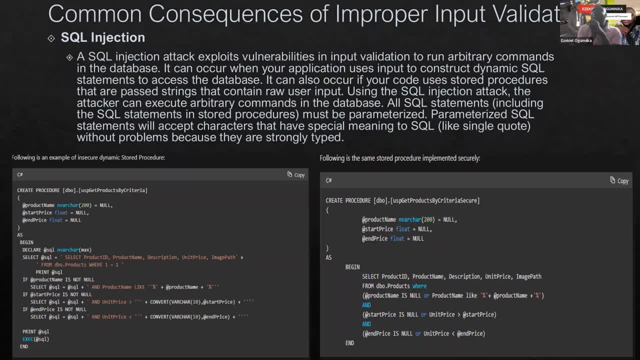 having in there. so using the sql injection the attacker can execute arbitrary commands. the database, all sql statements, including the sql statements in stock procedure, must be parameterized. parameterized sql statements. we are set characters that have special meaning to the sql sql, like single quotes, itself without problems because they are strongly typed and this: 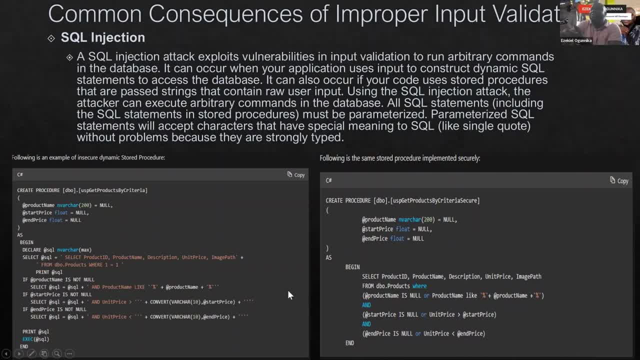 is one typical example of a stop procedure right, which takes a product name, of course, being parameterized, your start date being parameterized. but the downside to it is this is a dynamic- i don't know for those that are into the net- and maybe normal sql syntax as well too. 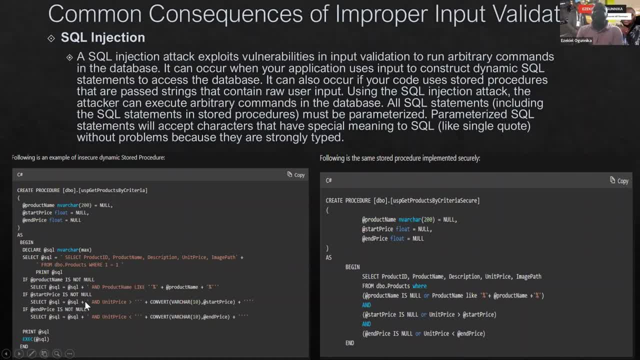 this is you having a purely trial uh xml itself written in text formed within the stop procedure, and you're running on execute syntax itself, which is always known as uh dynamic stop procedure itself. so you're constructing your text base with plain text and the light, and with these also the fact that you have a parameterized. 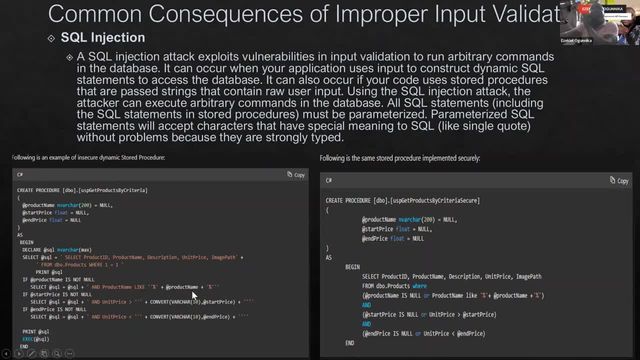 um variable. a possible sql injection is still can be carried out with this because you have your sql written as pure plain text. you know, within your text, within the products, just like the example glenn did, within your product name itself, um and uh, a malicious sql query can be inserted into the. 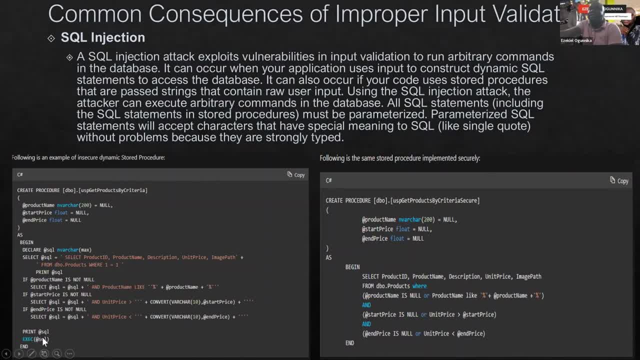 the product name itself. and by the time you run this last line called exec sql, you're not just only running your normal intended sql code, but you're running an injected sql query, rather, and which can really cause devastating damage to your, your application and according to um microsoft approach of getting things done. also, this is a 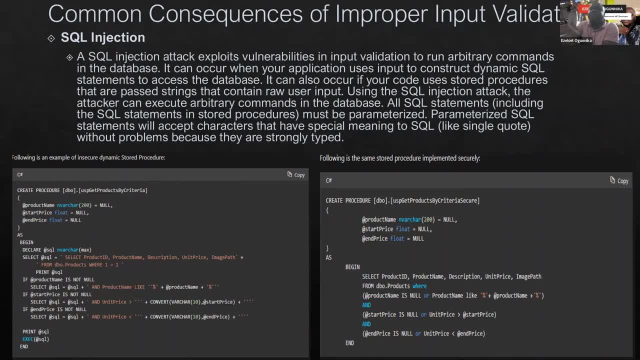 proper way of you running a similar same thing, same concept, same selection criteria, but in a proper way, without using the dynamic sql query. yet you can see it's still the same light, but this, culturally, uh, is way better than you having this execute. executing dynamic s stop procedures. 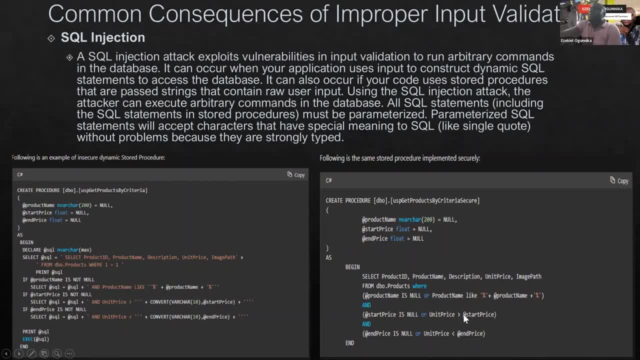 as it is, because this is actually more of like a strongly type and we'll do a lot of uh uh really, as SQL really accepts those characters that are within the context of SQL itself, and any other one relating to you exposing some stuff would never be executed in this kind of approach itself. 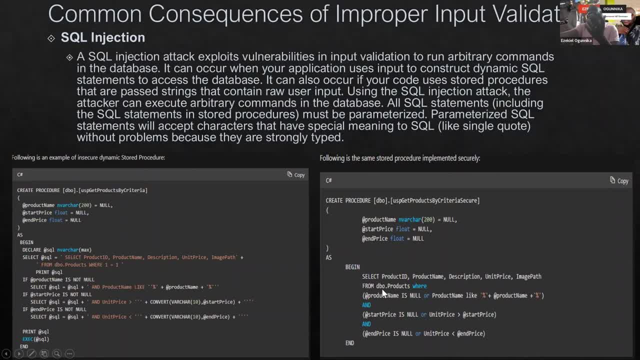 I know some of the security experts might say, oh yeah, with this we can still find a way around it, though, but, like according to Microsoft, this has been proven and it's been tested, and it's been proven to be very effective as well too, and so, with that being said, also right for we as 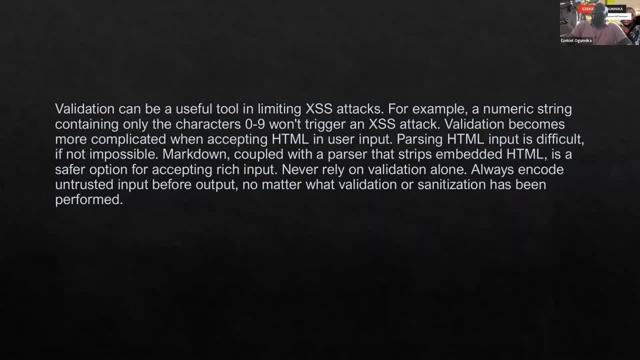 developers right doing validation. it's kind of very, very, very. it's not something you can just think of on the fly, think through. maybe because of a year of experience you can get it like. the framework Glenn talked about is also one very good place we could get use these tools also in trying 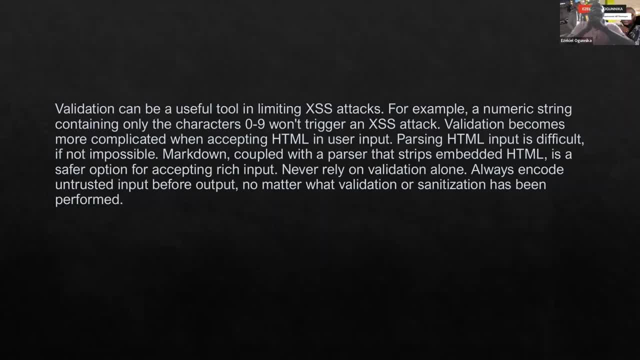 to test our applications and see how they so validation can be used, can be a useful tool in limiting data. for example, a numeric street containing only the characters of zero to nine won't trigger unnecessary data. validation becomes more complicated when accepting html in user input. passing html is: 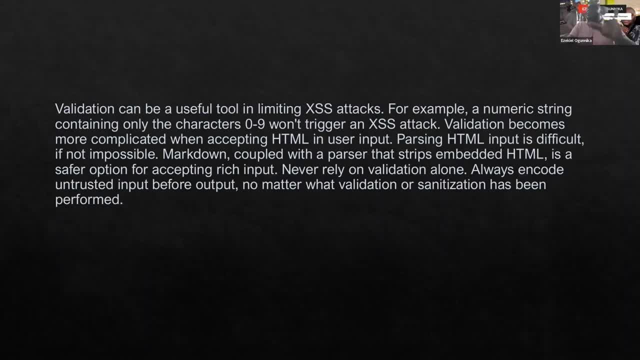 difficult, if not impossible. markdown coupled with a password that strips embedded html can be used is a safer approach for accepting rich input. never rely on validation alone. always encode untrusted inputs before outputting it, no matter what validation or sanitization that has already been done on your application itself, and the general practice is that encoding usual. 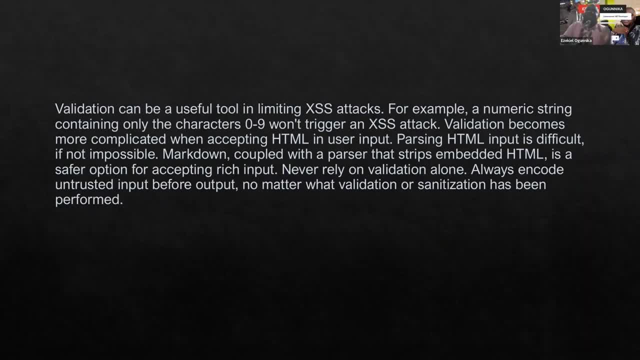 inputs is not a good way to do that and the general practice is that encoding usual inputs takes place at the point of output and encoded value should never, ever, ever be stored in a db. you understand, and the fact that during the encoding right, when you are encoded at the point 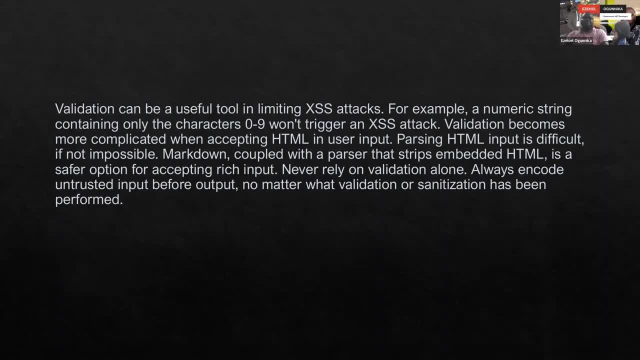 of output. this allows you to change the use of data itself. you know, for example, maybe looking at an html uh to a string query value, for example, without having encoded values before you search and allow, you can take it your, your. some of the bugs can take advantage of any changes. fixes you. 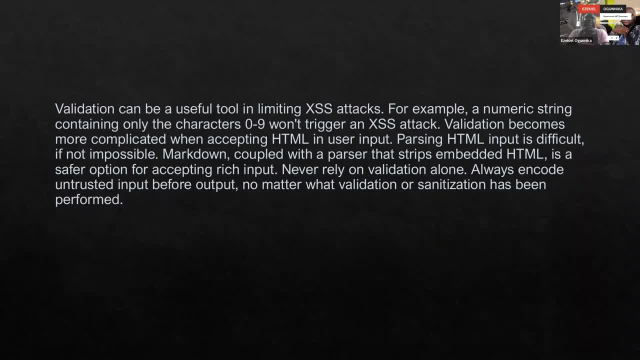 know, made to those encoders and they can actually exploit your system and they like so. for for me, i feel, um, when you, when we talk about simple validation and certain information, this lies more because an attacker like for we as developers, it's our responsibility to ensure that. 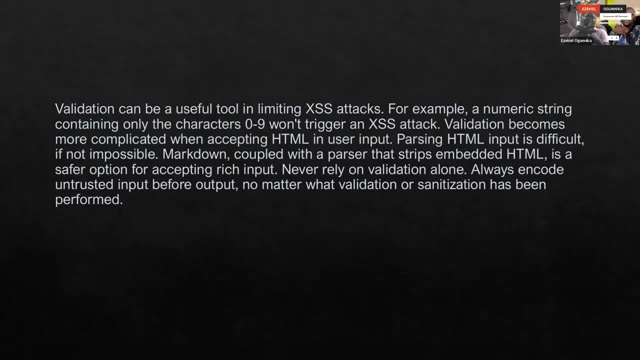 we, we spend more time in ensuring that, uh, the best we can do is what we are doing in terms of validating an input, and the best we can also do in terms of rendering this same data that we have already back to the to the user is also being properly done in the right way. 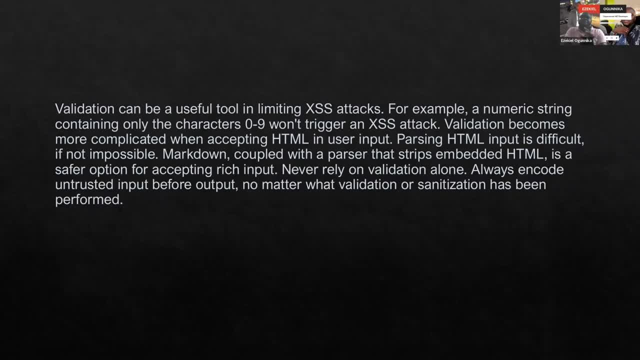 so i also protect the user and, like i said earlier, uh, the very first form of protection in any web application, any system, is from the source code itself, is from the, the application itself. then, before any other form of vulnerabilities can actually um set in, uh, like i said, i i 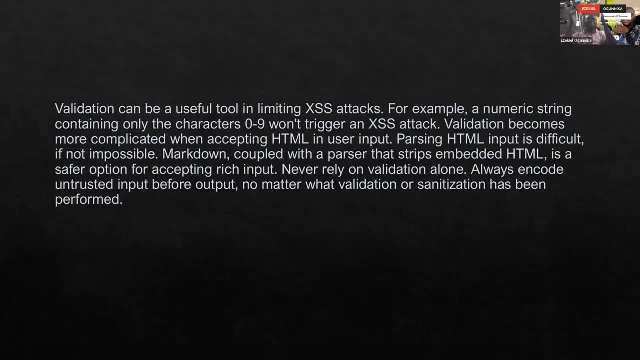 if i have to talk much on these, i think it should just be like going over what and what every other person on this call has actually said most actually, i keep making reference to glenn um tool and, like i said, this is one very important tool we can. 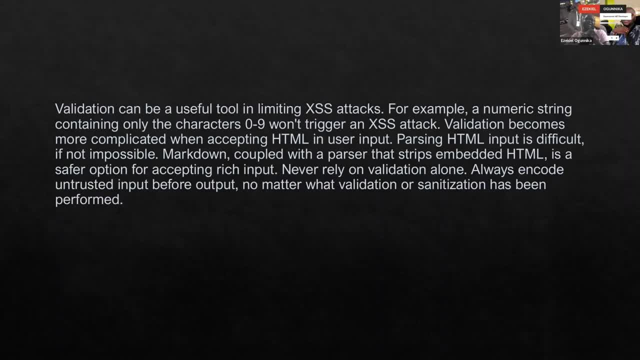 actually use uh as developers, you know, to check. there are several vulnerabilities that you can think of. these few ones that are chosen are just common that we know of. but lately, that's as the technology advances, also attackers also uh, they, they are by the day. they are also innovating. 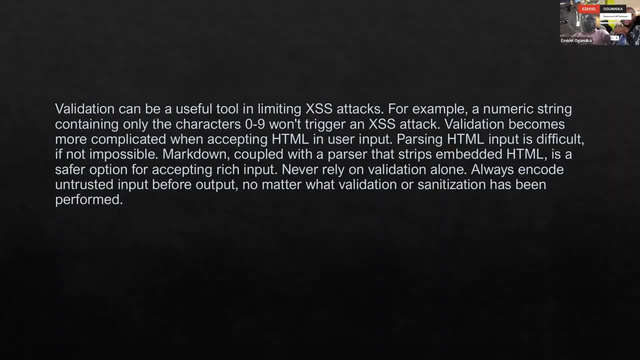 you know, trying to look at vulnerabilities and also, uh, from the angle of uh, martin, also uh, you have the dev up environments in your system running fine, doing your c rouge, your build pipeline are running, but like your dependencies itself itself, is anybody checking? you're using the. 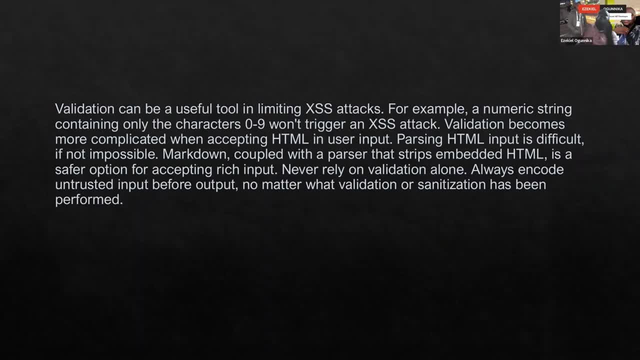 version of uh, maybe dot net framework 2.21, uh 2.2, for example, that microsoft itself doesn't even support. that myself said this is out of support if they have vulnerabilities within those applications. the rest are sure, microsoft is not going to release any patch, but within your organization you still have your key core concept, your key core. 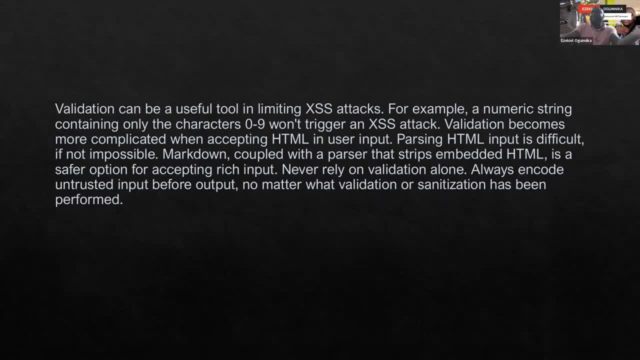 applications running on those frameworks. you know that's more like setting a house on a, putting the house on a on a light fire, that that could really explode anytime. so, like when we talk about security, input validation, data validation, uh, devops, and you know people basically, and people. 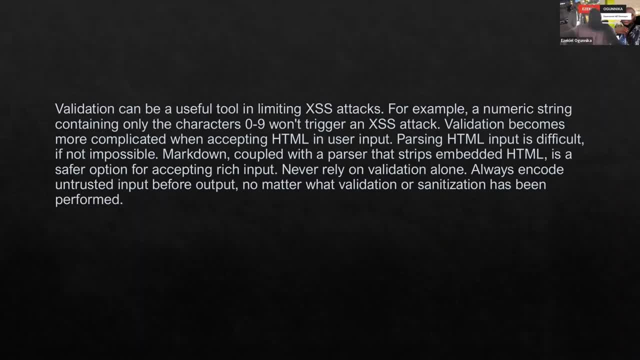 the process and, in fact, of course, the technology itself and the things we actually require in having a proper or a more secure environment. so it doesn't just lie with us as a developer. also it lies with the process, which these days, uh, uh, devops engineer, comes in as a developer, so you? 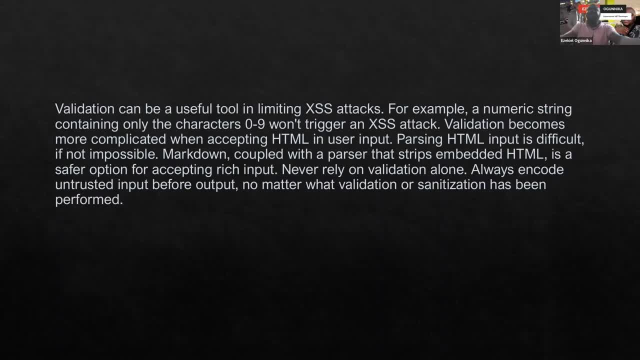 should also be thinking security. don't just think process, don't just think get shipping my code to uh pipeline. having a proper redundancy, having a proper contingency plan, is what makes a proper develop. security also is also very important. and uh, finally, just to round up what i have uh lined up for today: 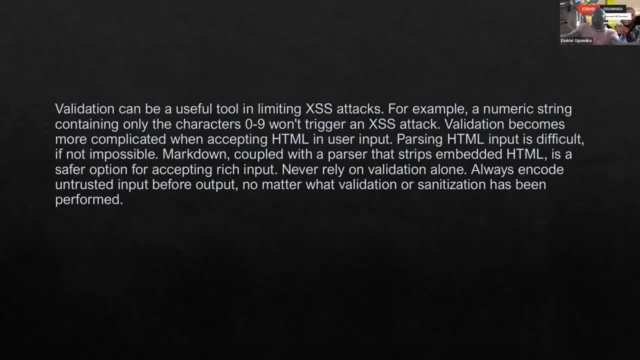 is also the fact that we can't do this alone, and that's why efforts have been made in having tools that could help us as developers, in doing lots of vulnerability availability tests as well, too, and i think the all apps are actually doing great also in setting up the right standards. 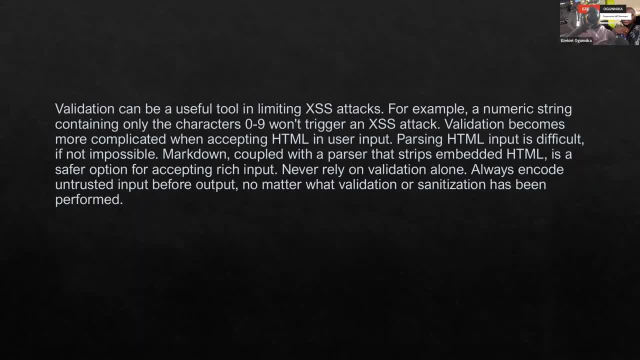 and where you can actually go check things before you push out your application to the your production environment. run them against most of these checks. see how you're doing in terms of improvisation, in terms of sanitation, how exactly you're doing and in terms of processes also how. 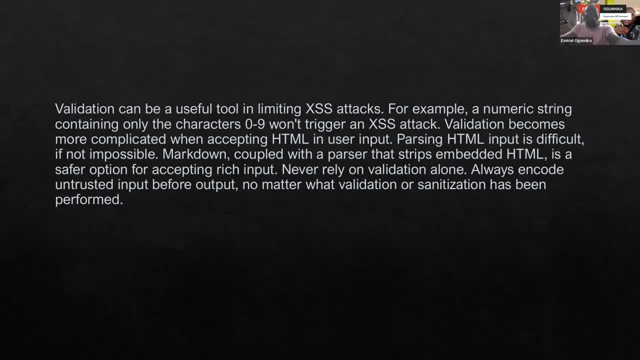 exactly are you doing as well too. so i feel at this point, uh, without taking much of our time, uh, this is my little presentation on input validation and data sanitization, and i really appreciate your audience and i would like, if there's any q and a at this point. 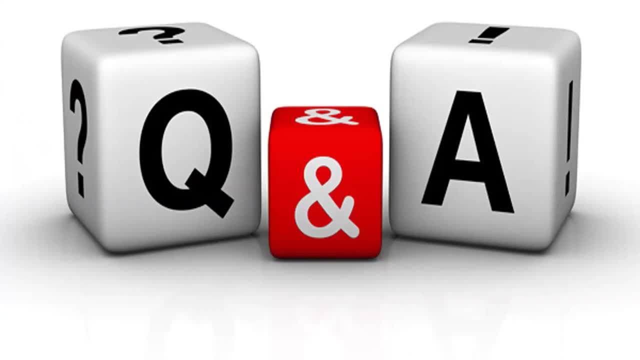 yeah, thank you very much. this accused. that was awesome, that was an awesome talk from you. and do we have any questions from the audience in respect to the validation and sanitization? because i equally agree, most times, uh, uh, developers and developers are always, uh, very reluctant. you know, by the time they start, the process starts to progress and things can slow. 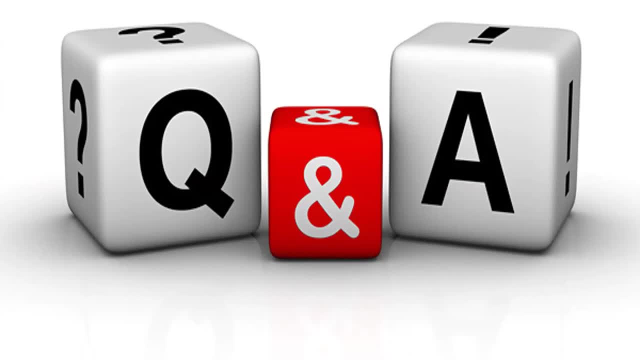 they start, they fix, uh, functionality issues. we now start telling them we have security issues to fix the highways in lockdown, that i've seen experiences on that, so all they care about is the functional aspect. so now, uh, bringing it together with security issues for them to fix, they they. 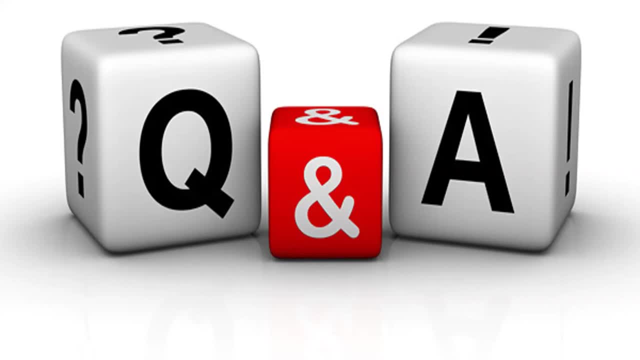 always see it as, uh, another task, a big task from the part. so i it's just a matter of balancing things. you know, most times they always want someone to come in to assist in respect to that. but if they have that back of their mind, just as, as you've said, pushing your course to ci cd. 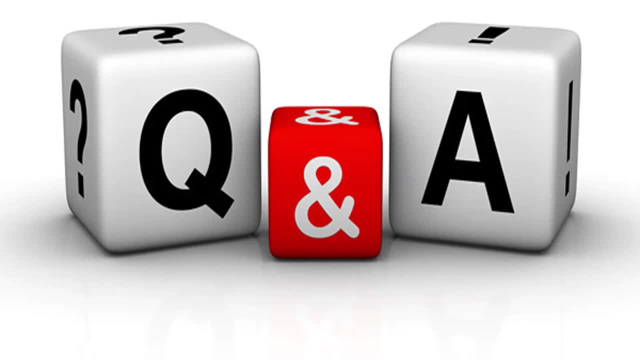 you must, even from the stage of uh developing your course, there must be security in me so that you you keep checking it even before pushing your code. by the time you check it, it will go a long way in uh giving you a clear status of our security. so thank you very much, ezekiel, for. 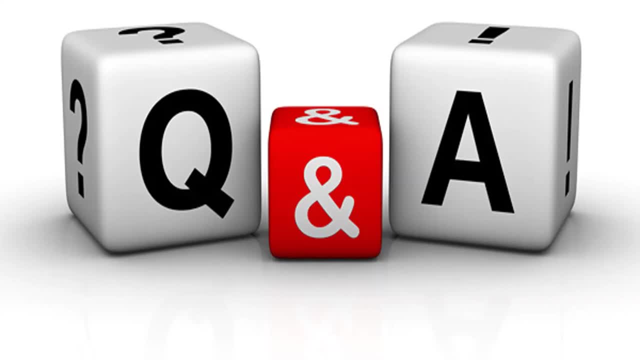 coming for this event. there is no question on ground for you and we hope that we never will call upon you next time you answer us. what time is it there in canada? uh, this is 11: 20 here. still, uh, morning here. yeah, yes, yeah, we are. we are in the afternoon here, so thank you very much for. 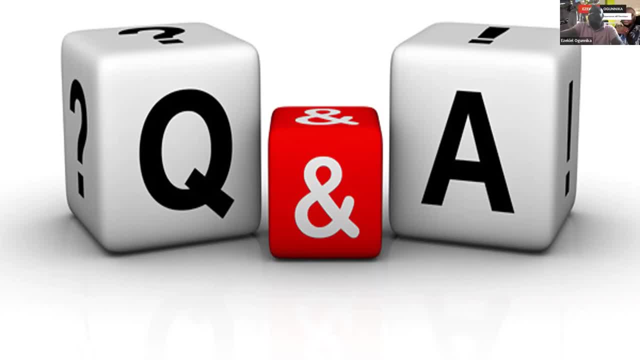 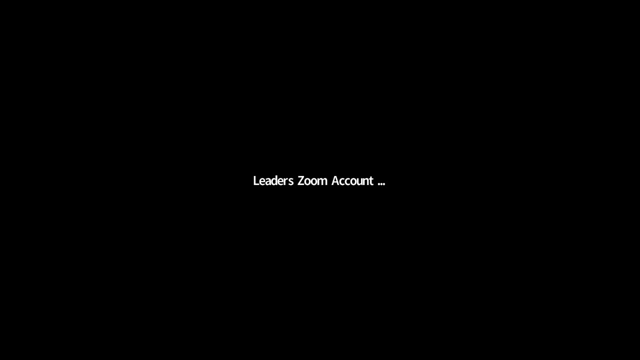 uh coming on the program. thank you so much for having me around too, and it's a pleasure meeting uh great minds um all on this call. thank you very much, so greet your family and greet your friends over there, thank you. so this way we are going to be cutting uh the events. 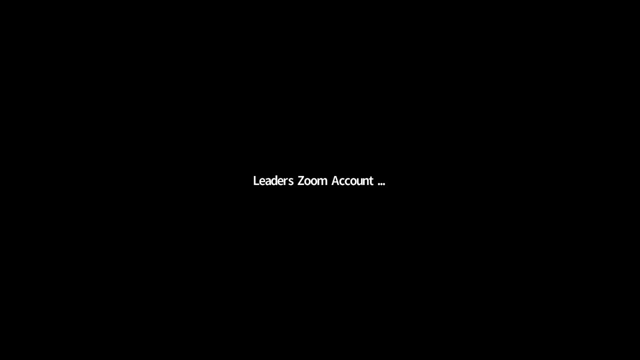 for today. we thank you. thank everybody who comes around. despite the fact that this weekend some of us needs to rest, we still have our time to be on the program and events today. so, um, if you need any slides, you can drop your email. i'm going to forward the slides to you. 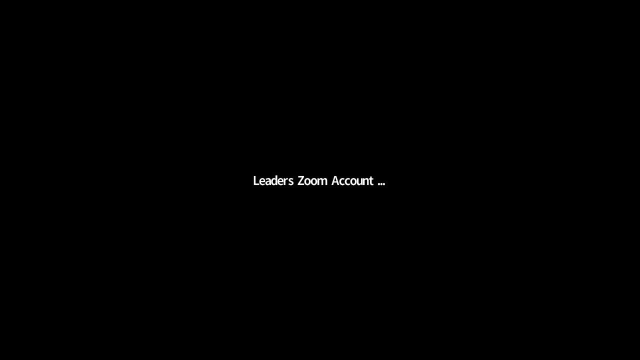 later on and, uh, you can keep up with the, with the community and the program as well. so, yeah, so i hope you enjoyed today's event and i'll see you soon. um, if you have any questions or questions, i'll answer them. i would like to hear from you, so please do share them with me. and if there are any comments about any of the events you're using, we still have time to be on the program, on the event, so, um, if you need any slides, you can drop your email. i'm going to forward the slides to you later on and you can keep up with the community. 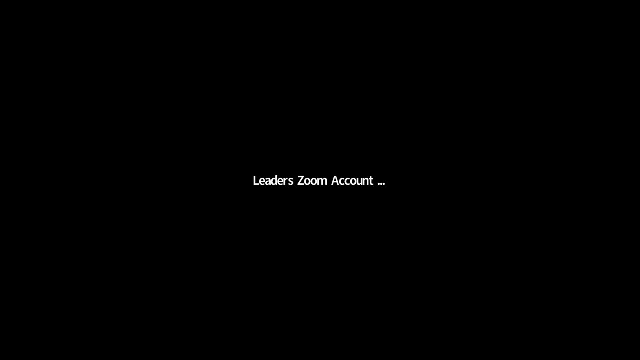 as we will be dropping one or two information in respect to OWASP, So I'll be dropping the WhatsApp group and also some necessary details on the chat now, So you as well can drop your email in case you need any information, So that one will be passed across to you.